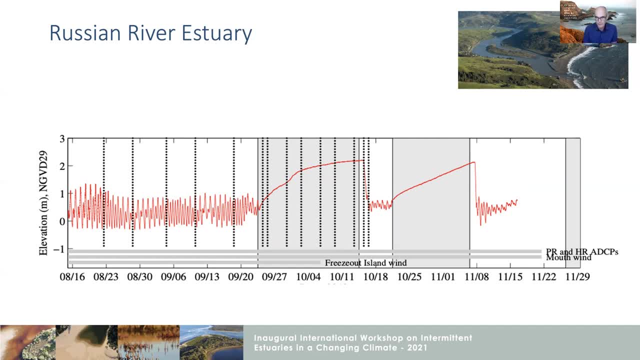 tidal variability and then, when it closes the gray area, with the increase in the in the water level, the black line- I mean the red line- going up and then asymptoting a bit as you get a water balance with high water levels in these closed systems where the inflow can be balanced by water losses. 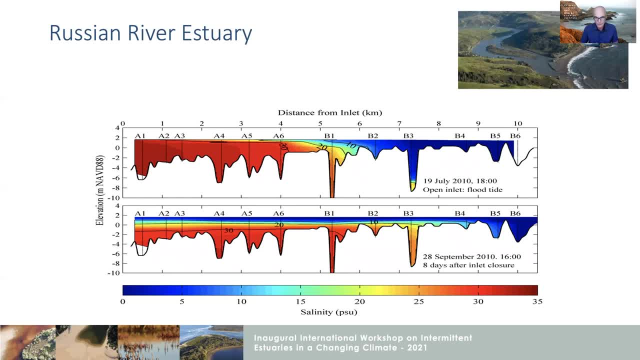 What the thing? that the other thing happens dramatically is that the top is a is a change to stratification and the top is a longitudinal salinity gradient: from red near the mouth- high salinity- blue and near the, the, towards the land 10 kilometers up which is low salinity. 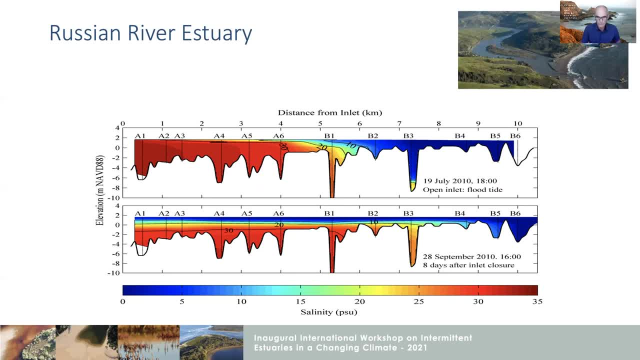 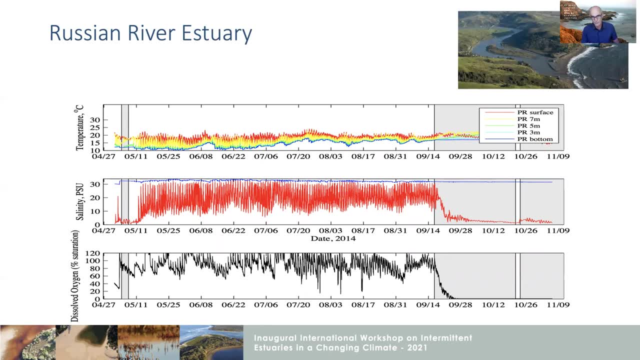 and then when the mouth closes, that longitudinal gradient changes into a vertical gradient. The other thing happens can be seen in this time series. of these two images Here you can see the lower one is salinity and the middle one is the frontal temperature. but middle one salinity, the lower one oxygen and particularly looking at the lower one, 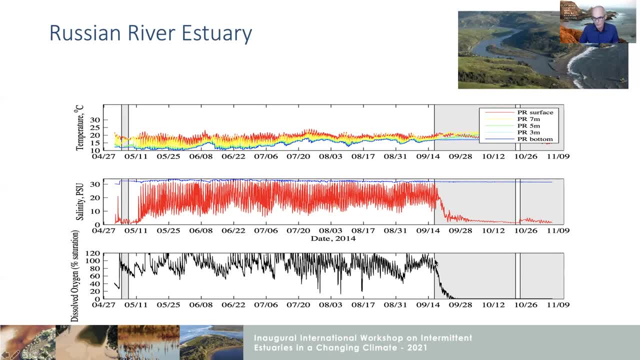 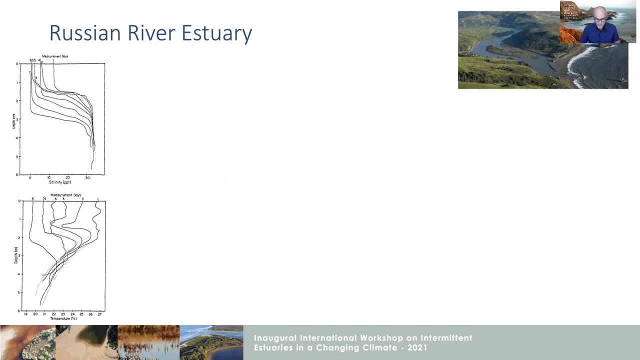 here the oxygen is is fine, around 100, varying a bit until the mouth closes and then drops to zero over a period about a week, due to natural biological oxygen demand, and this is expected and observed pretty much in most of these viable test juries. strong stratification is remarkable and- and i'd like to illustrate it with this data- that 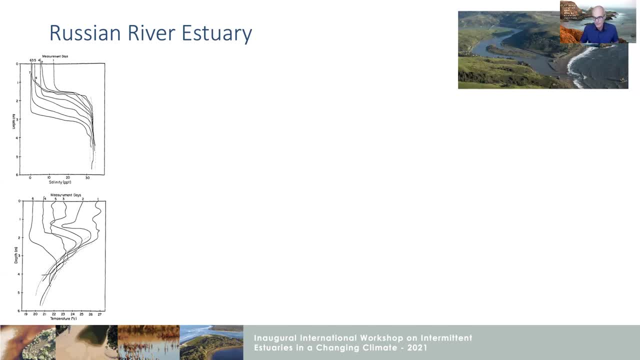 joe slinger and i collected in 88 in palmetto stream, south africa, the top one being salinity, bottom one being temperature profiles. over about a two month period and you'll see this bottom water salinity barely changes and likewise the bottom temperature barely changes. so this bottom 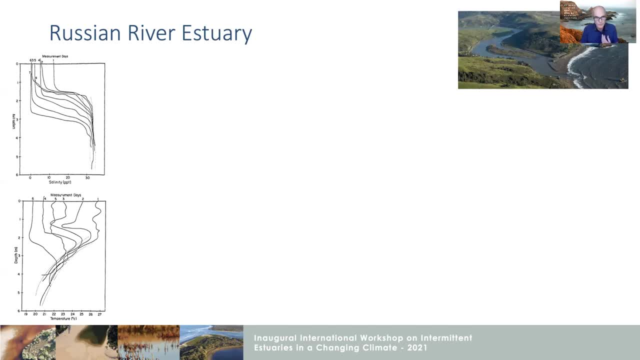 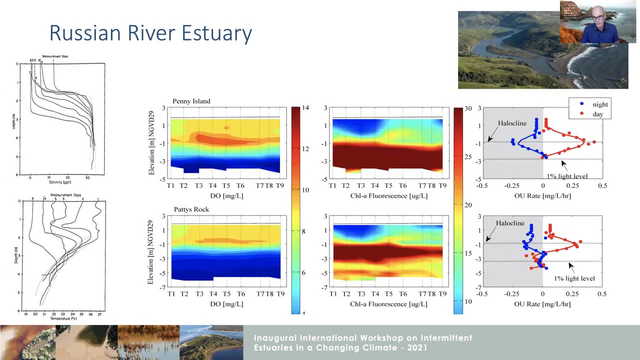 the. the rate of vertical diffusivity is sort of molecular. basically turbulence is shut down. so we've looked at this in more detail in the in the russian river um. one site is penny island- the top three panels here and and the others patty's rock. penny island is near the mouth here. 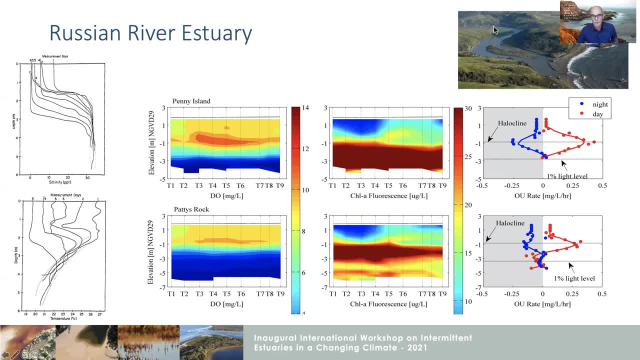 and patty's rock is is on the bend of the of the estuary and you'll see that patty's rock oxygen over a 24 hour period. the high oxygen actually hyperoxic in the um in the interface and hypoxic upload interface um and so using salinity data. 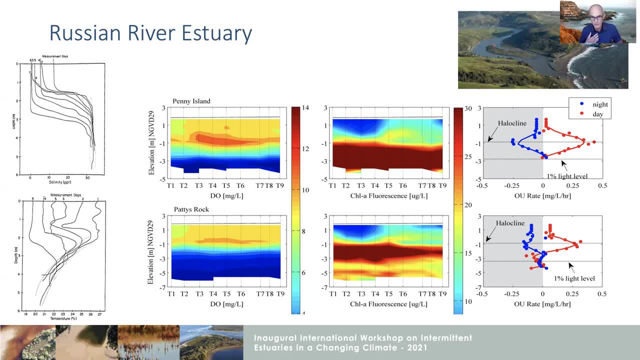 we could deduce vertical diffusivities and, knowing that using an oxygen balance, we can show both at patty's rock and penny island this red increase in oxygen during the day and decrease at nighttime due to photosynthesis and respiration in an interface or metal imian. 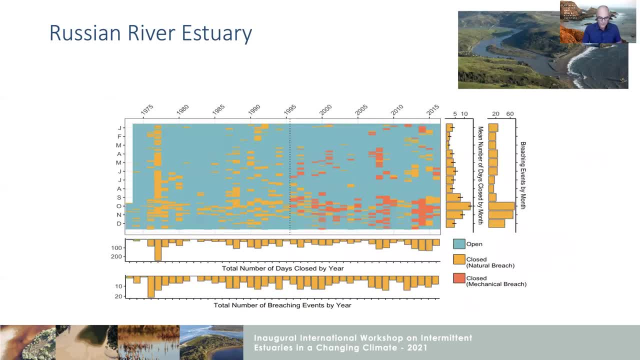 where there's essentially no turbulence going on. so when the mouth closes is not only important in relation to the river and the forcing of waves and rivers and tides, but it's also important to the consequences if it closes in the middle of the night, and it's also important to the 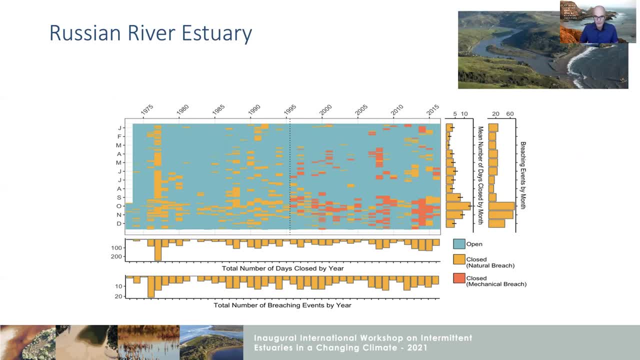 surface and the fall of the summer, shorter or longer days, more or less light, and also the surface warming, and this has turned out to be pretty important in the russian river estuary where we're looking at at habitat for steelhead trout. and this plot started with dane berenson. and katie dubois updated it and sam winter worked on it as well. um, over about a 40 year period. here you've got january to december, 1973 to 2017, and the oranges are the most commonly closed in october, november, december, which is late summer, fall, autumn, actually more. 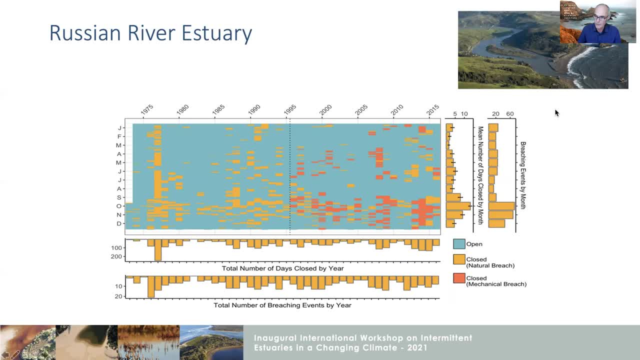 like early winter, to be honest. and- but not only that- monthly climatology, but you also have this inter-annual variability, with um it being more closed in some years than others, although since about the 90s it's been less, largely due to management and the climate change and the 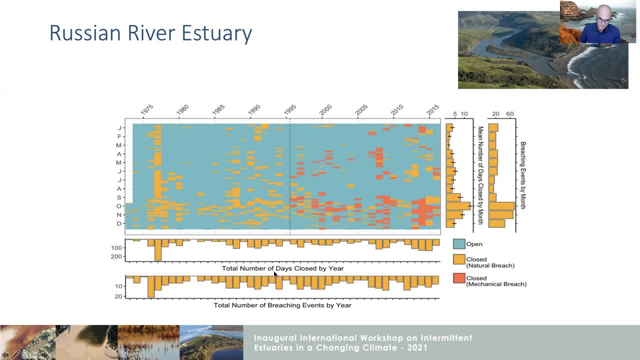 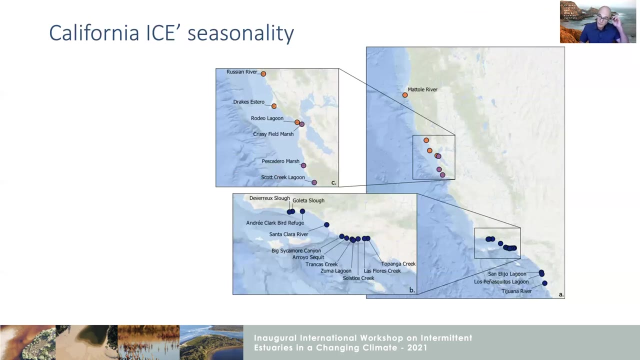 red is where the mouth is opened artificially. but looking back here, in 82 it's a very wet year, the mouth didn't close, and in 77 it's a very dry year, the mouth is closed much more than normal. so this work has continued through sam winter's masters, where he's looked at all these sites. 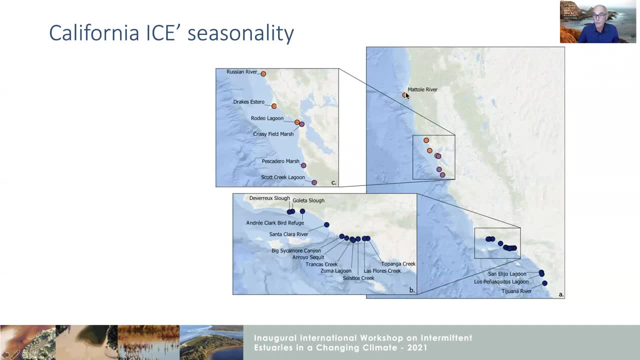 through california, from the more the wetter areas in the north mottola river to the dry areas in the south of tijuana, and identifying different seasonal closures. some close and some don't, some are some only closed in the fall, some close in the spring. but if they close in the spring, the 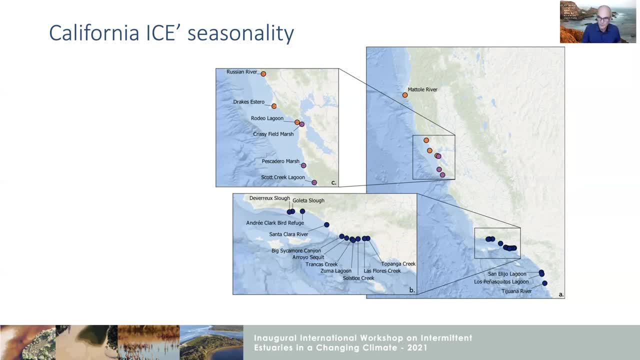 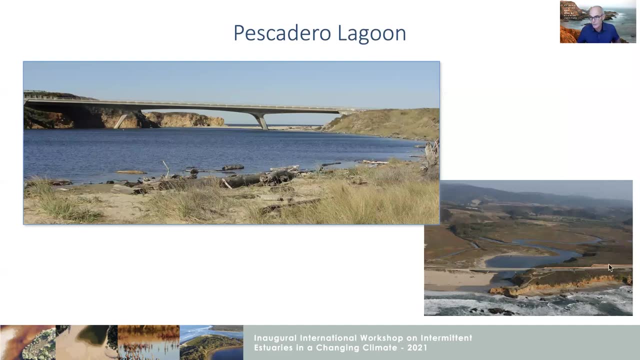 tents stay closed. but variations on the theme, even in the same climate climate region. so now jumping to pescadero lagoon, which you can see in the right here, it's much more like a coastal plain with extensive marshes, not like the canyon of the russian river, but in these channels, when the mouth 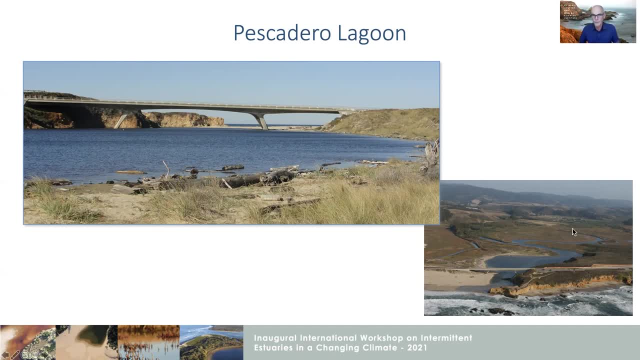 closes, you see the same, of course, water level rising, but also the same stratification. the rise in the water level is really important here because it inundates the marshes and that has impacts not on not only in the marsh, which is super important. uh, what will be addressed later? 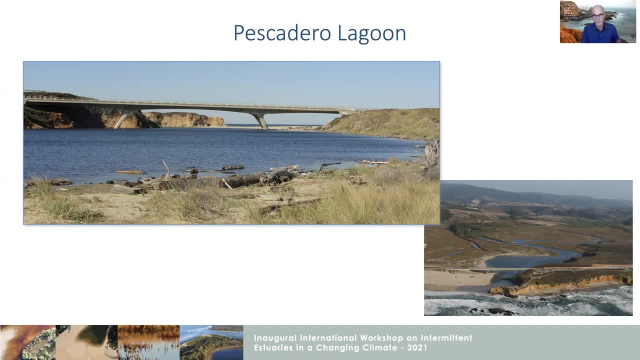 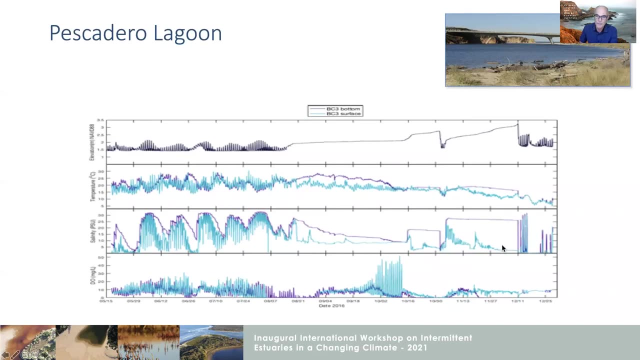 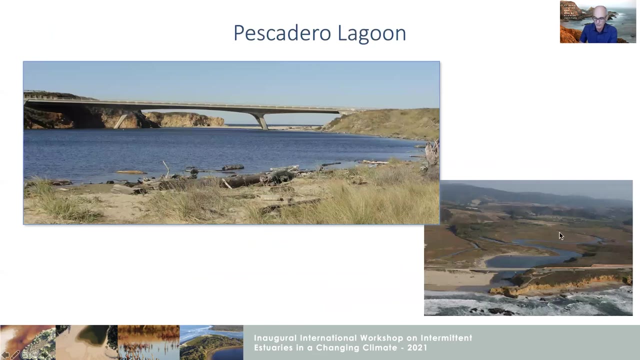 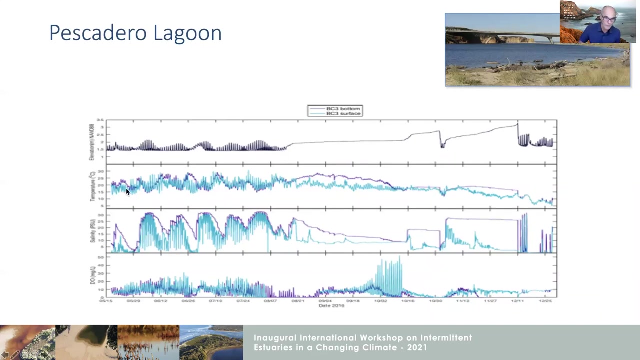 on, but also because the marsh channel connection becomes very important. so just one example is um data from may to december 2016: uh site bc3. so just going back, bc3 is up this channel, on the corner there, and you'll see a few uh things going on. if this is a water level and the top and the temperature at the top and the 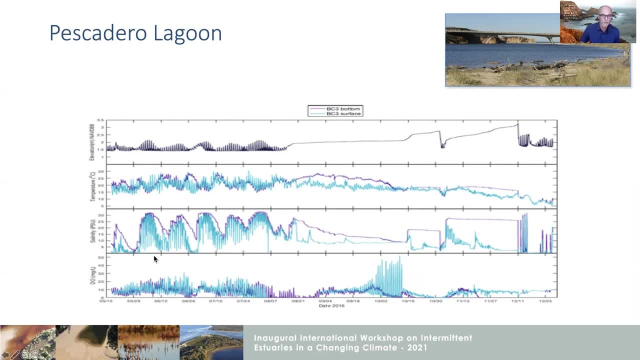 bottom temperature, top and bottom salinity, top and bottom oxygen. it's intriguing pulsing of the salinity, uh, and if you look up you can see the pulsing of the tidal range which basically lines up with the spring neap cycle, uh, which and dane behrens did show in russian river, but is really 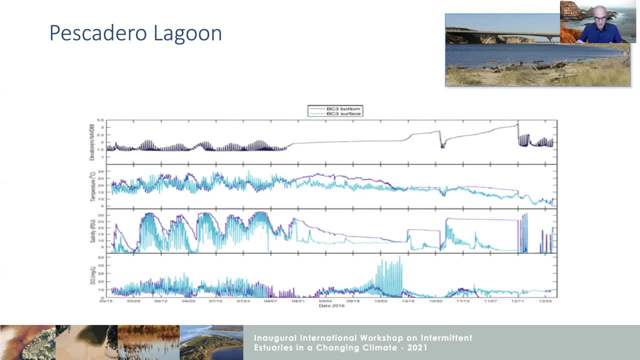 marked here in these smaller systems, how the mouth changes and pulses with it with the tidal range and with that the stratification from mixed to stratifies and with that the oxygen. but then you also see, here's the closed period. the water level becomes flat for a long time. then there was an 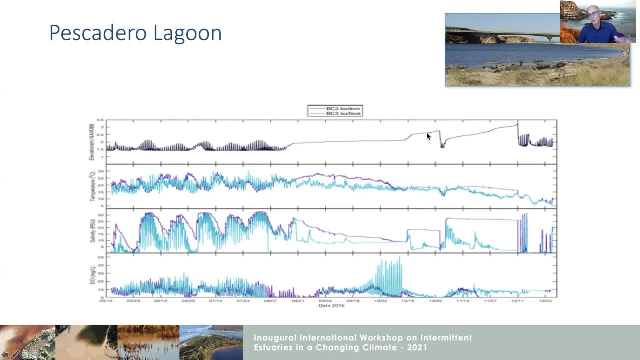 early rain in october and the water level went up just enough to crest over those marshes. and if you look down oxygen, you see that's when the oxygen crashed and what's happening here is not just the bottom, oxygen being low. so that's the russian river model which we see here in in august, where 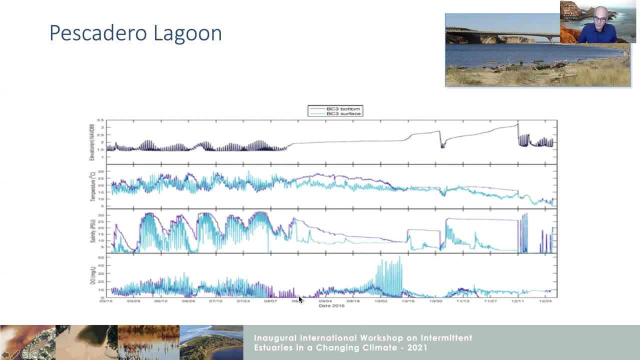 the top and bottom salinity is separate. it's not just as much as what we were looking at earlier: stratified and the bottom oxygen goes to zero. but this here in October is because the marshes are getting inundated and supplying a whole bunch of of crud. it's probably the best term oxygen demand. 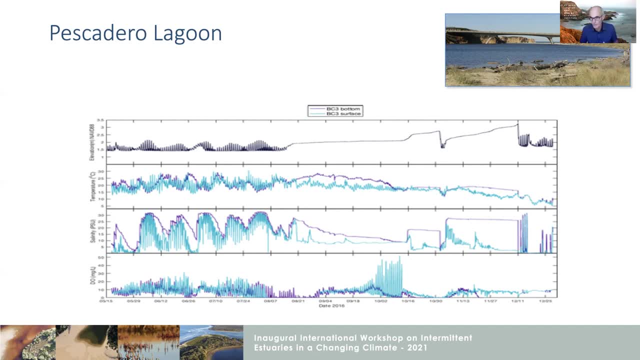 mostly reduced substances that strip oxygen really quickly into the channel, which reduces the oxygen and it's the worst during breach events. and so this system we started working on because whenever it was breached you tend to have a fish kill and this water would be top to bottom anoxic or close to it for days and the fish had nowhere to go. so pescadero has been a really 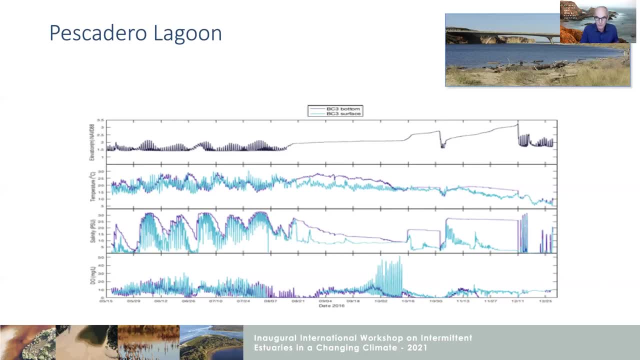 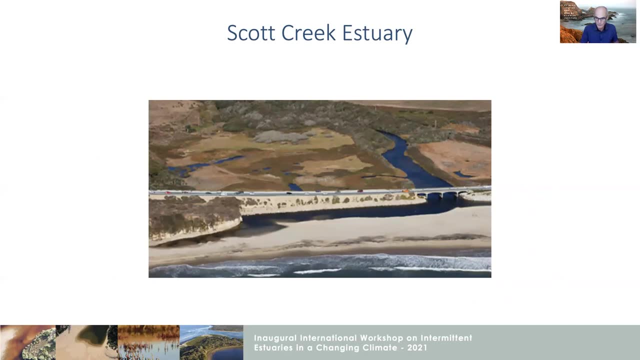 interesting study in the importance of marshes in these systems. and the thirdly is a contrast. Scott Creek estuary is is a really small perch system. if the mouth is fully eroded, there basically be no water in the system. and here we see shorter time scales and slight differences, big differences. due to that. Daniel Nyland at his 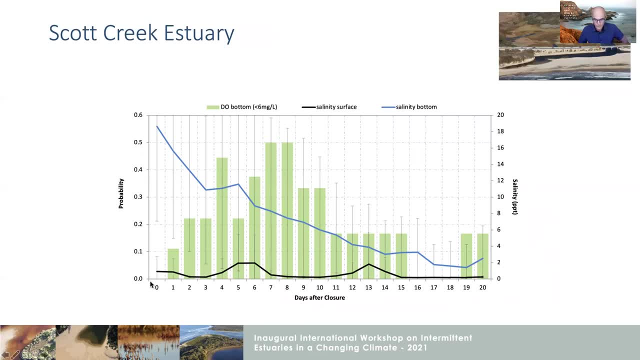 masters here and what we see here is, if every closure he made time 0, the day closed and then this is a plot of 20 days. and when it closes the bottom salinity is high- this blue line- but off over the time it gets lower when it closes. there is no oxygen impairment really, but these green. 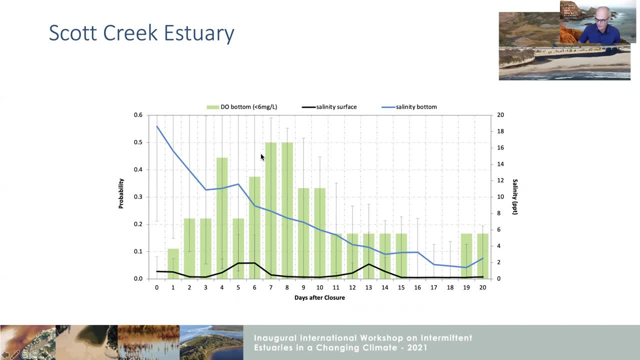 bars are the probability of oxygen being less than six milligrams per litre, which is critical for um for fish. and it gets worse, worse for about a week, which is the same as a Russian and a few other places we've looked. typical natural BOD will kind of do that. but then it starts getting better again and it gets better. 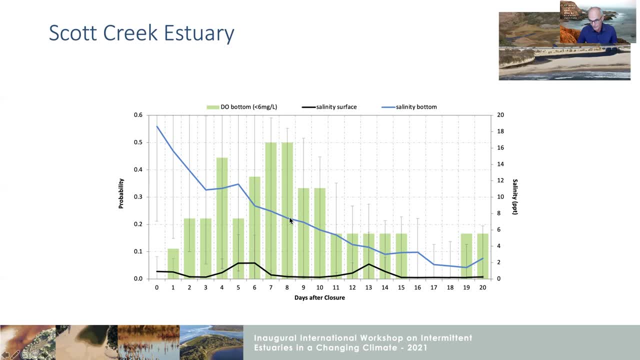 because the salinity at the bottom is is dropping. it's basically the bottom layers being eroded out and it's very much what we saw in the palme, not in that deep section I showed earlier, but in the shallow section. the bottom layer gets eroded. the hypoxia doesn't last more than some. 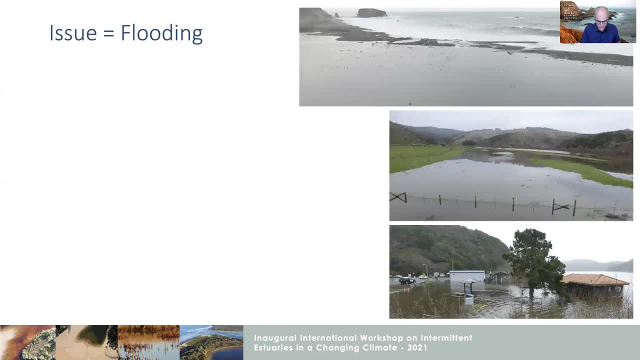 days. so the key issues that are driving a lot of this research and that we need to address as scientists, to help you know, guide a guide: management of these systems. the one is flooding. here's the russian river. when the early winter storm built the berm higher than normal, they 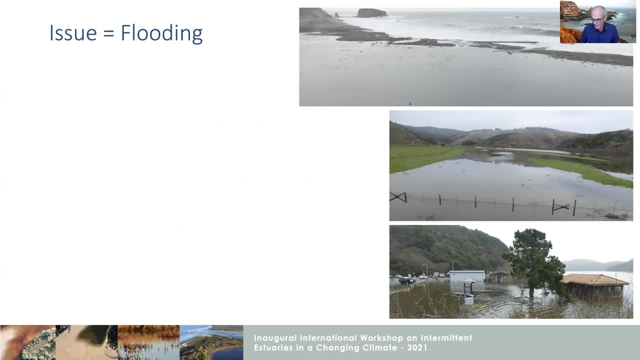 couldn't open the mouth, so it flooded naturally and flooded the natural floodplain which happens to be this: the town where the of jenna and across the coastal highway and the mart and the and the farms. these are natural systems where we've developed the floodplain, just like many other. 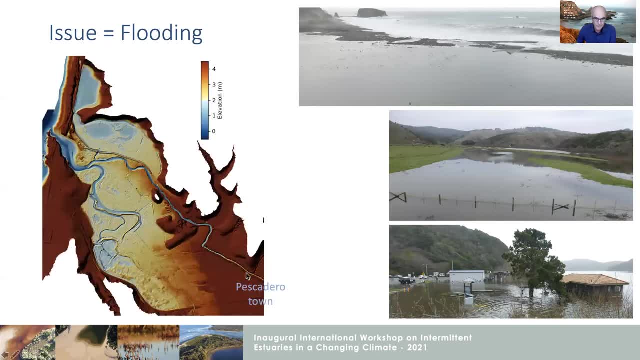 river systems and a pescadero is kind of, um, like this picture of digital elevation with the creeks coming in and the marshes and then the town's built in the floodplain. yes, it's above the tidal marsh, but not much, and it's flat because there have been previous times when it flooded and 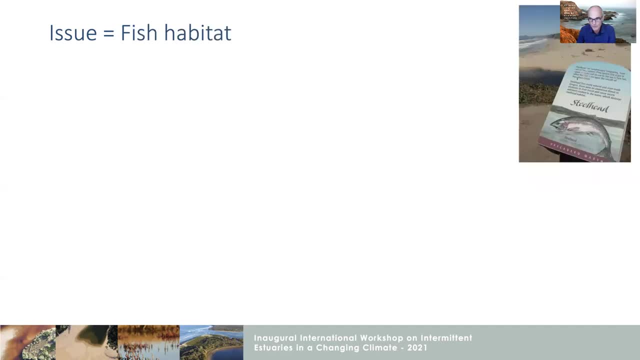 flattened the place out. secondly, a fish habitat, steelhead charter, one of the most common, but coho, chinook as well, and um, over here, we, we, um, my slide's not advancing for some reason. there you go, so over here we have looked at water quality, temperature, salinity and oxygen. 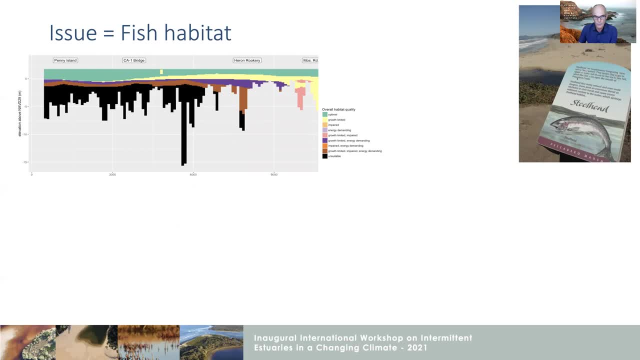 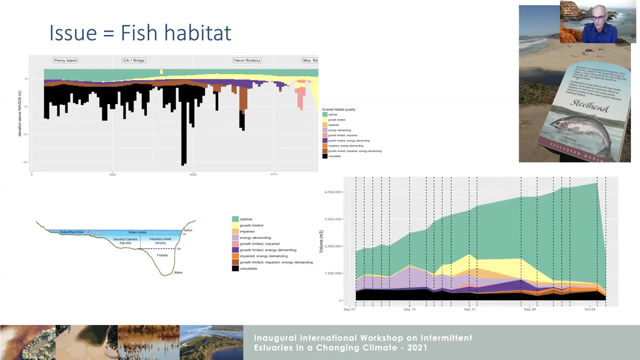 and created these longitudinal sections in the russian river and showing black being unsuitable because of oxygen. each of these categories is different depending on temperature, salinity and oxygen. the green is is the best, but we also can track it through time over here for about two months in in 2013 and you can see. 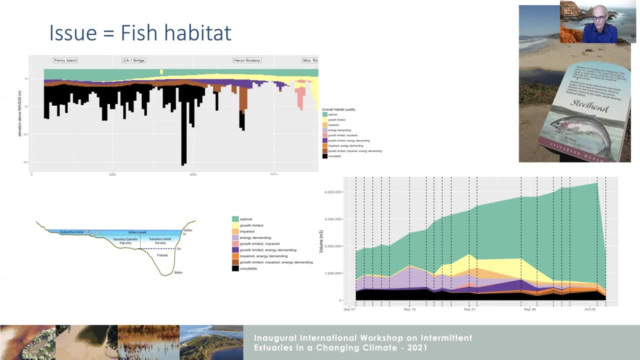 the green- uh cool low salinity layer growing through the closure and the black layer sort of getting less but not really going away. but it's small compared to the others. so we're looking at the different pressures on on the habitat driven by warming on the one hand. 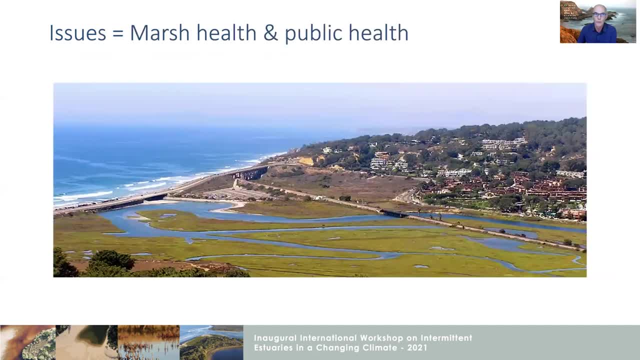 by ocean intrusion on the other hand, by stratification, hypoxia in the third hand, and then the last issue, then, is marsh health and public health. so the link between the closure and the hydrology and the marsh marshes need to be inundated, not to desiccate, and the marshes need 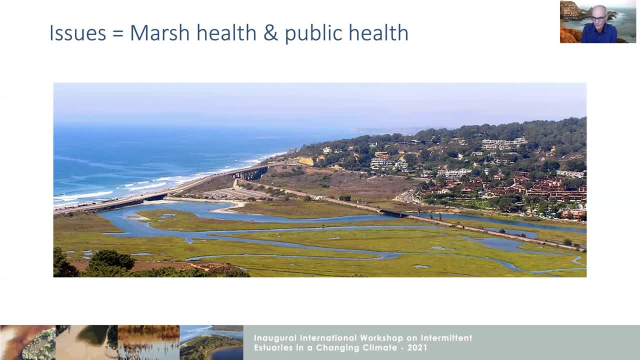 to be inundated in order to accrete, so this is something you're working on. a sea level rise is: if you want marshes to keep pace, you need them to accrete fast enough, and the public health thing then is: is effective mosquito control when mouths are closed in the big freshwater wetlands they 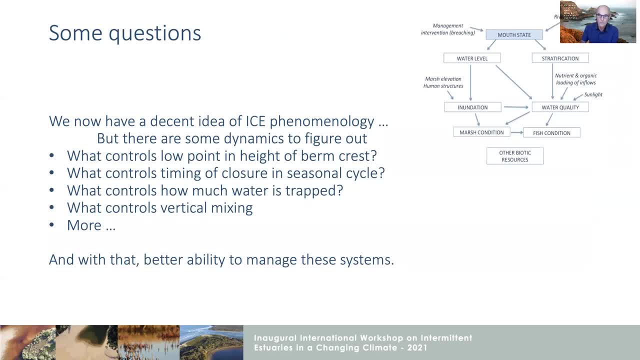 harbor mosquitoes. so some questions just here to uh think about, about the questions we need to answer about what controls the low point in the berm, what controls the closure timing? what controls how much water is trapped? what controls the vertical mixing? these are the science questions that we have to um, that we have to figure out.